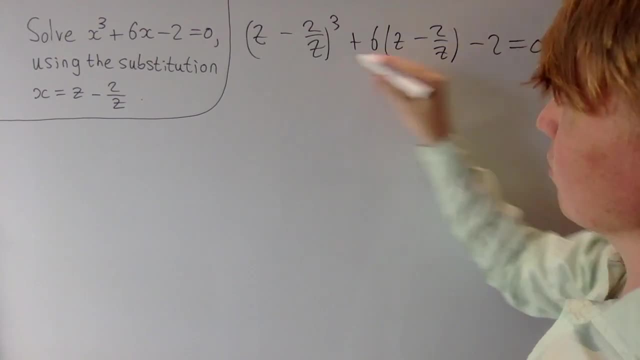 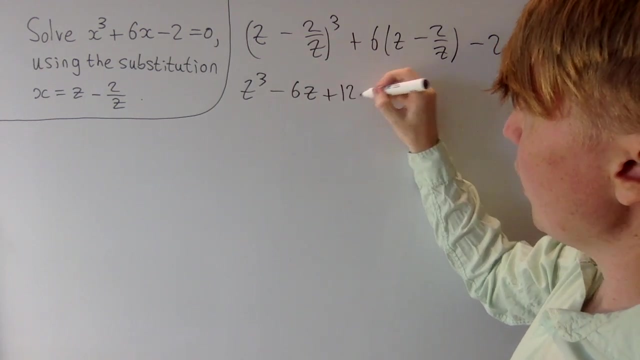 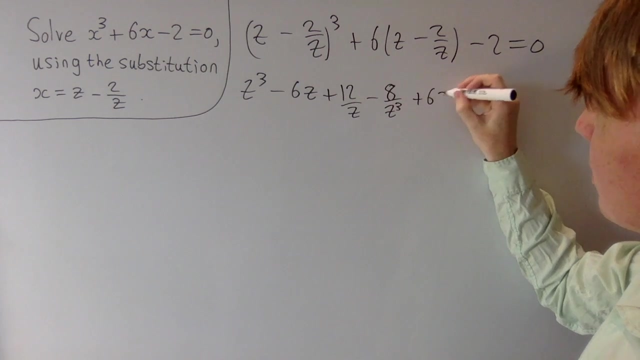 and tidy up and see if we can solve to find z. So, expanding this first bracket, z cubed, we get minus 6, now just times z, then plus 12 over z and finally minus 8 over z cubed. when we just expand all of this Then we also get plus 6z and a minus 12 over z from here. 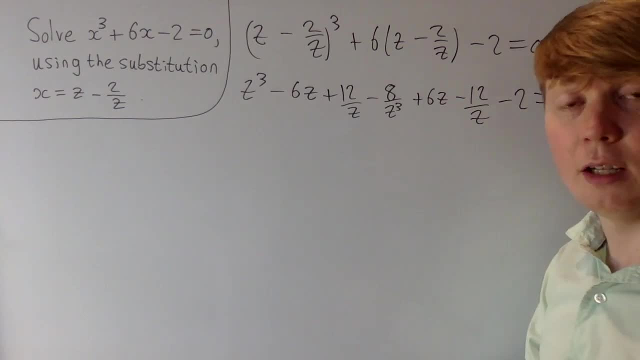 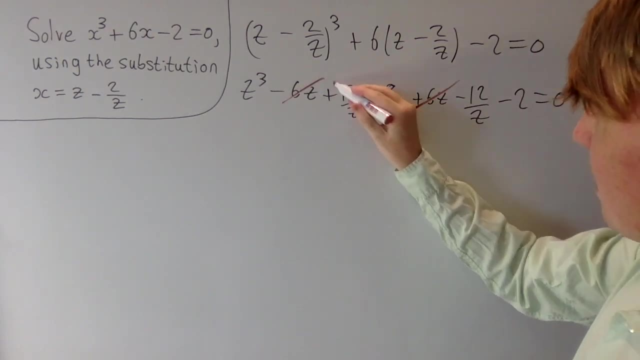 finally with a minus 2, and then all of this is equal to 0.. So you'll see here quite a few things are going to cancel: Our minus 6z cancels with our plus 6z. We're going to have a minus 12 over z and our plus 12 over z cancels with our minus 12 over z. So this: 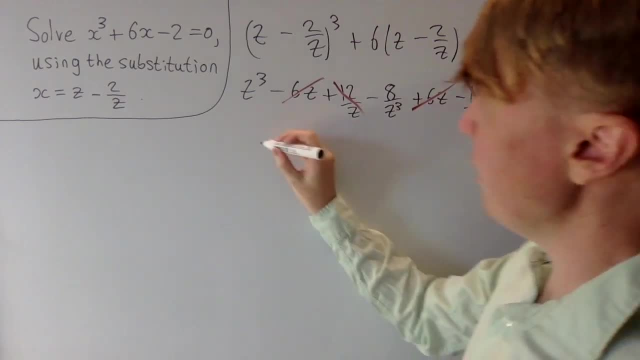 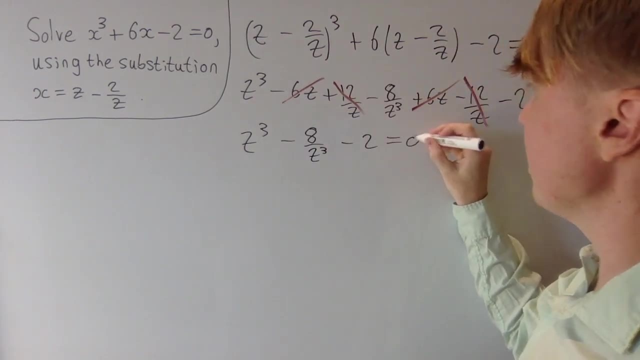 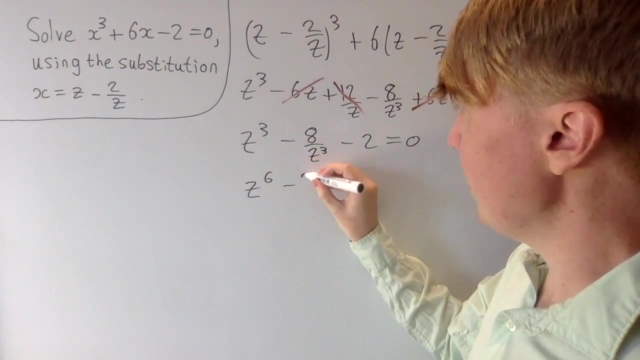 reflects the substitution choice we've made there. So now all we're left with is z cubed minus 8 over. z cubed minus 2 is equal to 0. And what we can do here is we'll multiply by z cubed, So we get z to the sixth. then we'll write it as minus 2, z cubed from the. 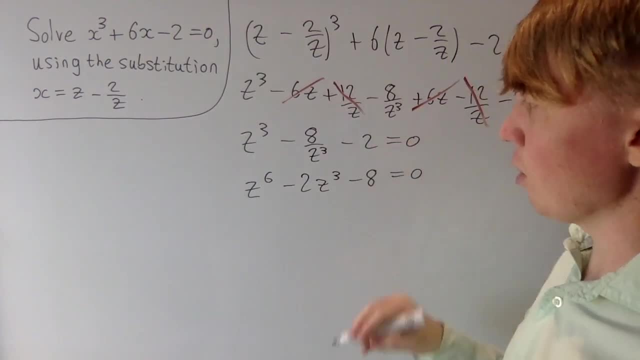 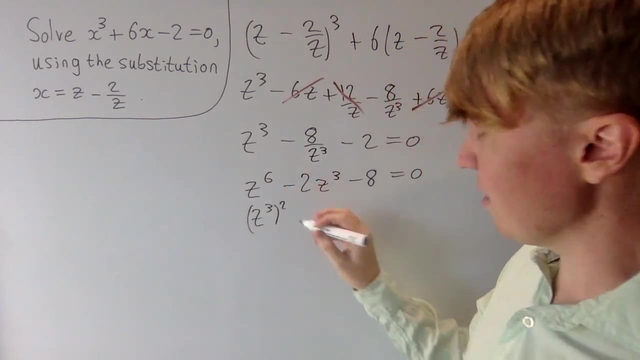 minus 2 term minus 8 is equal to 0. And it might not look like we've simplified things very much, But this is actually a quadratic in z cubed now, So we can write z to the sixth as z cubed. 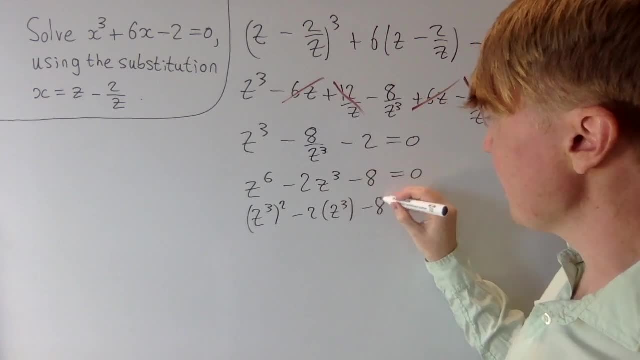 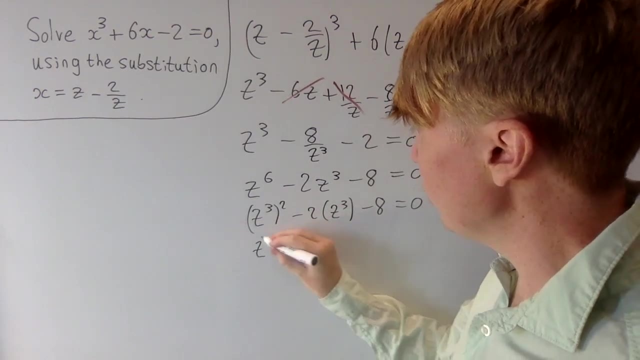 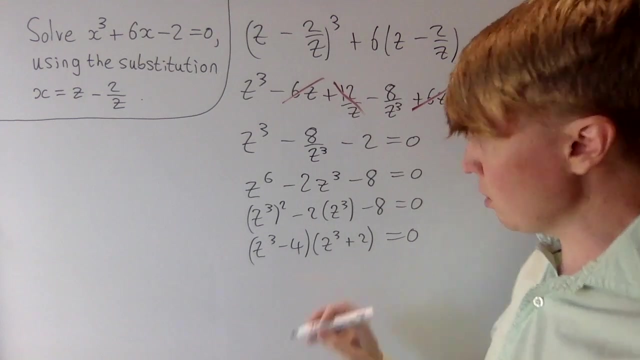 squared minus 2, z cubed minus 8, and this is equal to 0.. So this is now something that we can just factorise. We get z cubed minus 4, multiplied by z cubed plus 2 is equal to 0.. So we see here that our solutions then are going to satisfy. z cubed is equal to 4. 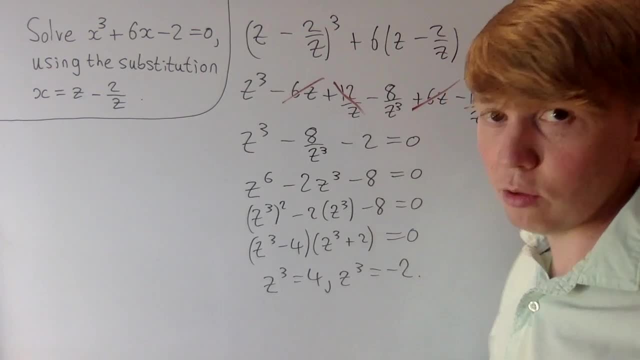 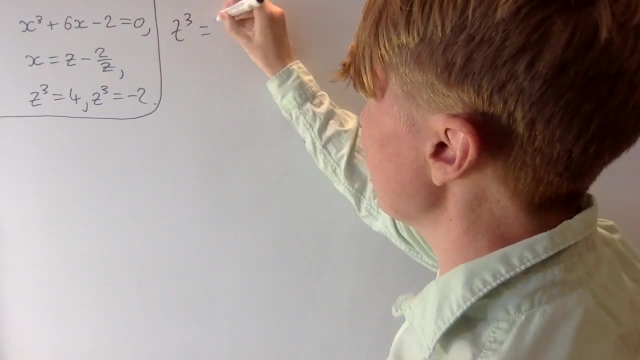 and z cubed is equal to minus 2.. Now we can find our solutions in z. So when z cubed is equal to 4, we can just take cube roots and you see that 1 of our solutions is going to be: z is the cube. 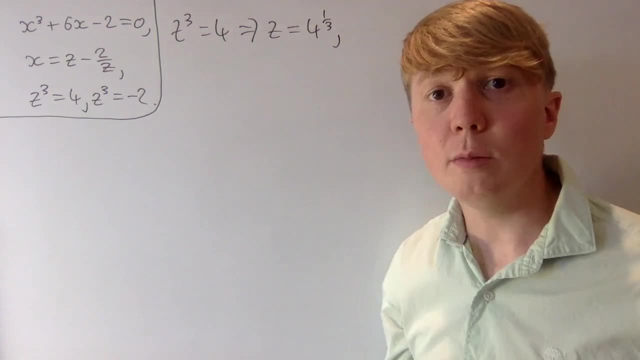 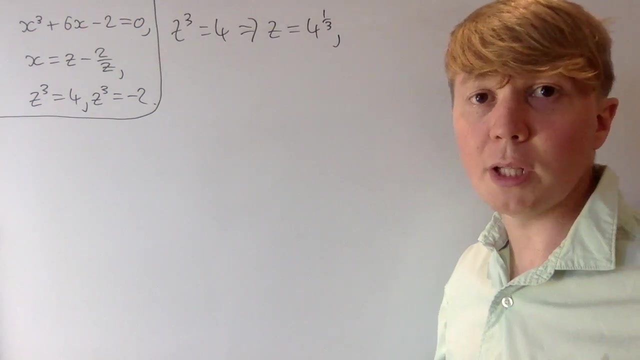 root of 4, or 4 to the power of one third. But this isn't the only possible solution if we allow complex solutions as well. So here, instead of just having 4 to the power of one third, we could also multiply by any cube root of 1.. It's the cube root of unity. 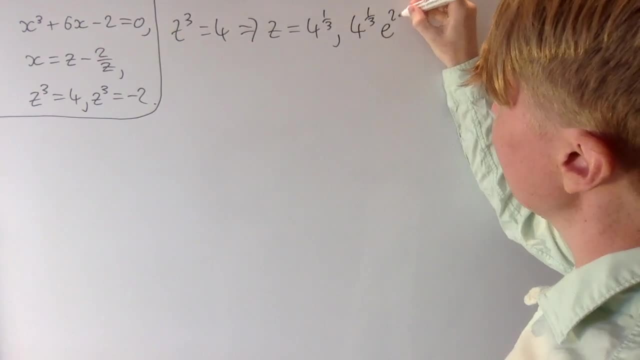 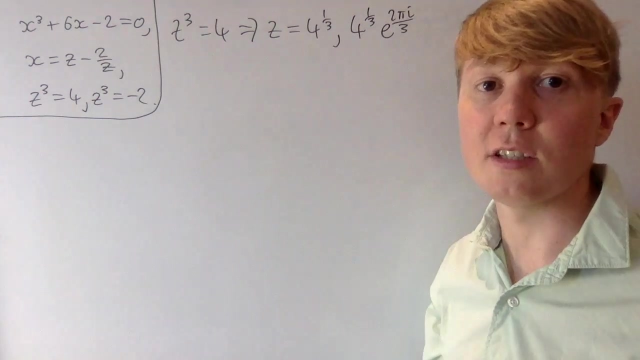 So we get an extra solution 4 to the third times E to the 2 pi i over 3, where if we all of this, you get that to four times one. so this would indeed be a solution to z cubed equals four. 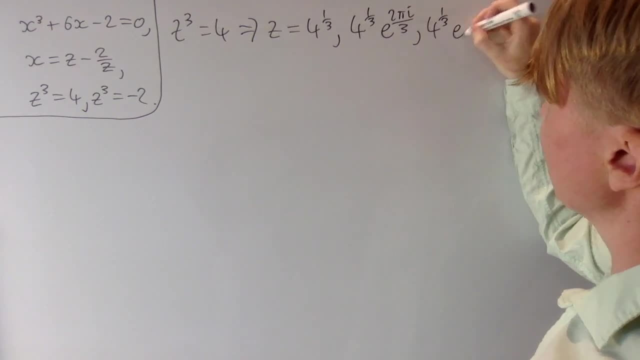 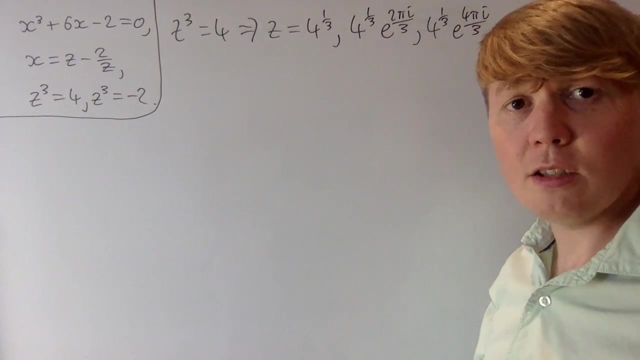 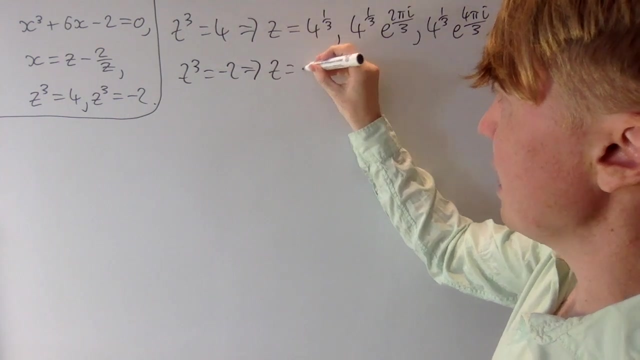 and similarly for our other cube root of unity. you get four to the third times, e to the four. pi i over three would also be a valid solution to z cubed equals four. so now let's do the same thing when z cubed is equal to minus two. our real solution is just going to be: z is the negative. 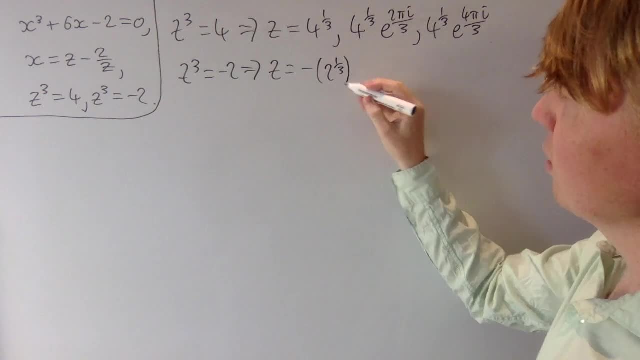 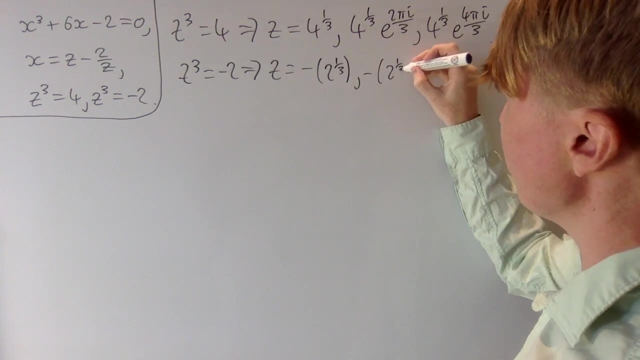 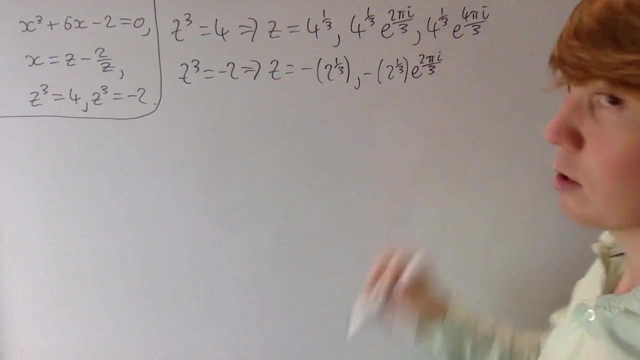 of- i'll put this in brackets- the cube root of two. so this is our real solution. we can do the same thing again where we multiply by cube roots of unity. so minus the cube root of two, multiplied by e to the two, pi i over three. when we cube all of this we get back to minus two is times one. so 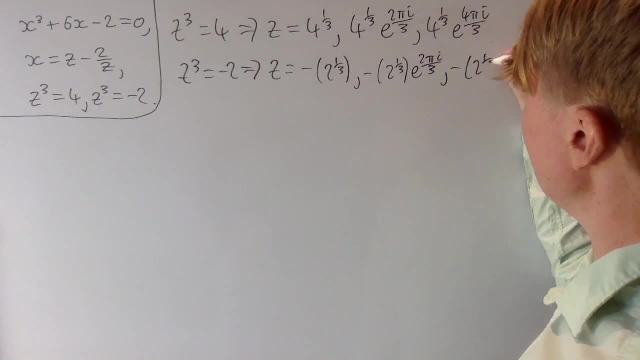 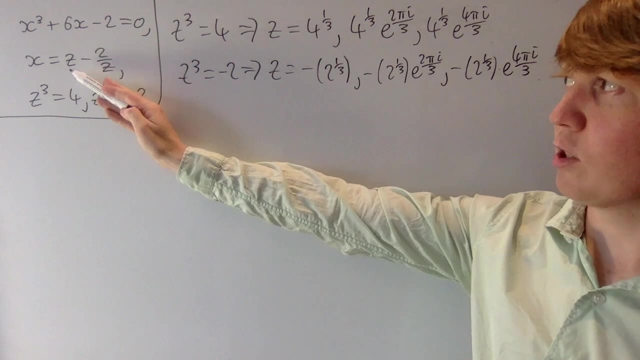 this is a valid solution. and similarly for minus the cube root of two times e to the four pi i over three. so we're about to substitute these into this expression: z minus two over z. so just for convenience here we'll rewrite our fours as twos to the power of two. 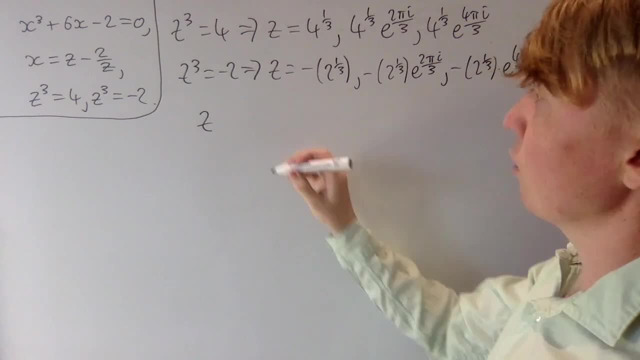 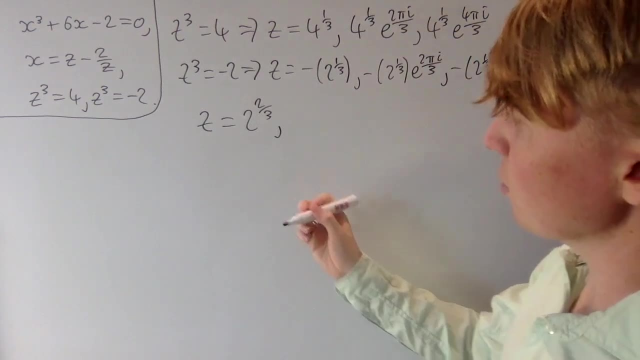 so what do i mean here? we'll just write z instead of four to the power of one third. this is going to be two to the power of two thirds, and we'll do as well with these cube roots of unity. we'll introduce another letter here, so we'll just say that w. 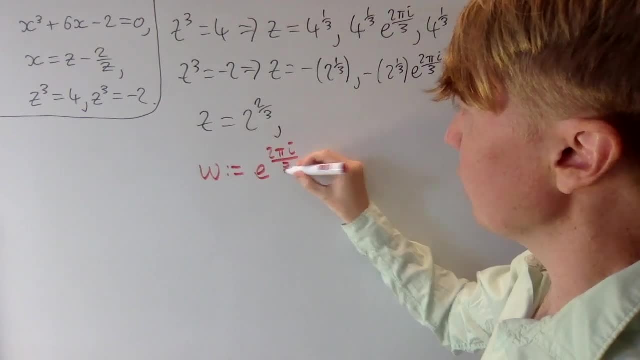 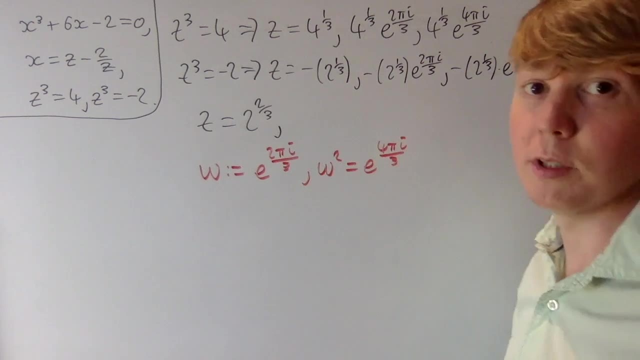 is going to be e to the two, pi i over three, just for convenience, and this is nice, because then w squared is equal to e to the four, pi i over three and w cubed is just equal to one. so this gives us a nice way of expressing all of our potential solutions for z here. 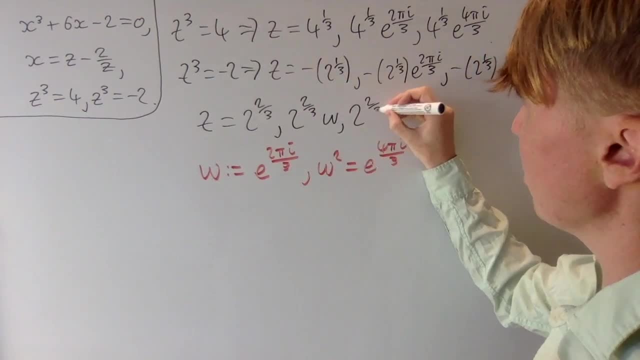 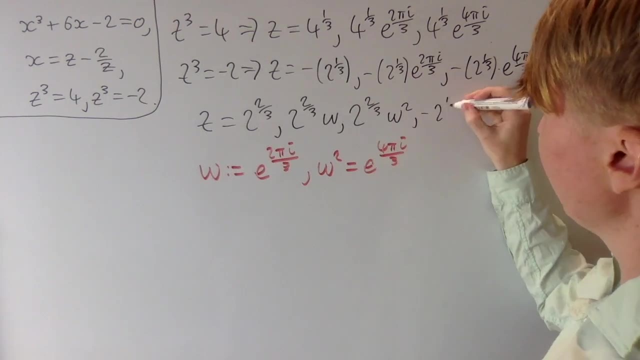 two to the two thirds times w. you've also got two to the two thirds w squared up here. then we get minus two to the one third where we don't really need the brackets there, and also minus two to the third times w and finally minus two to the third times w squared. 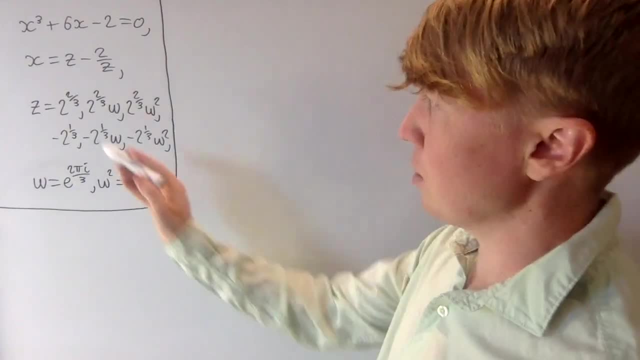 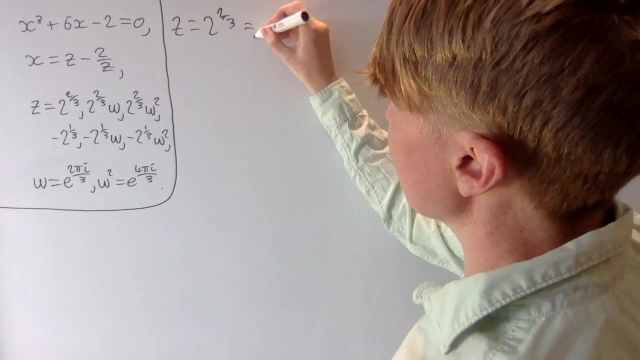 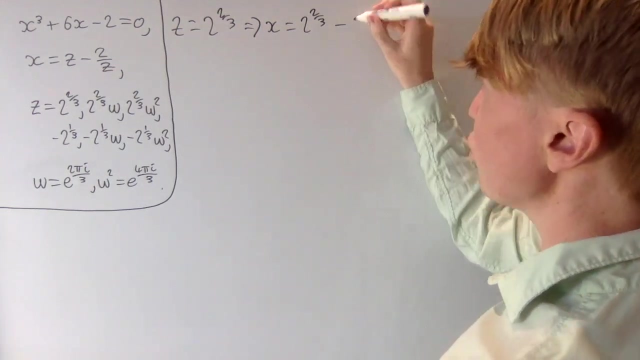 now we can substitute in these z values to find our x values. let's start off when z is two to the two thirds. substituting this into z, minus two over z, tells us that x is going to be two to the two thirds, minus two over two to the two thirds. so minus two to the power of one third. 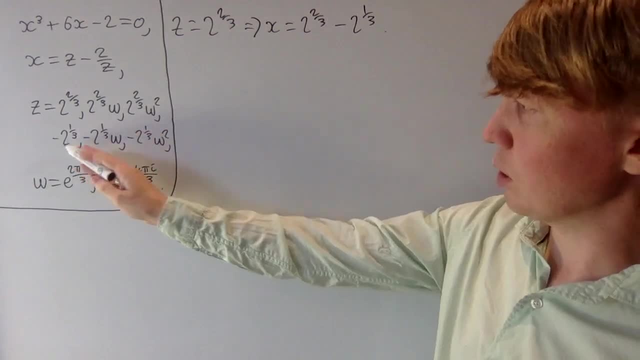 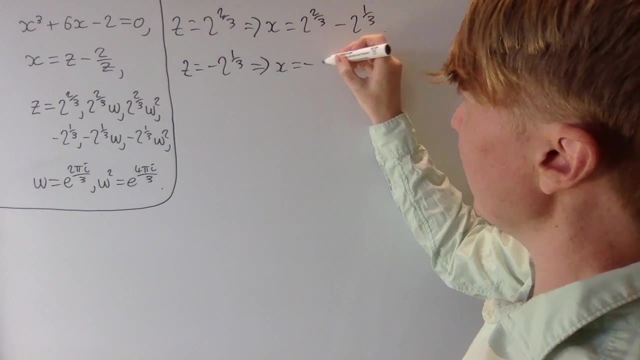 is our first solution for x, that we'll start with the easier one, so we'll go on to. z is minus two to the third. now what this tells about x? well, x is going to be minus two to the third. then we do minus two over minus two to the third, so we end up with a plus two. 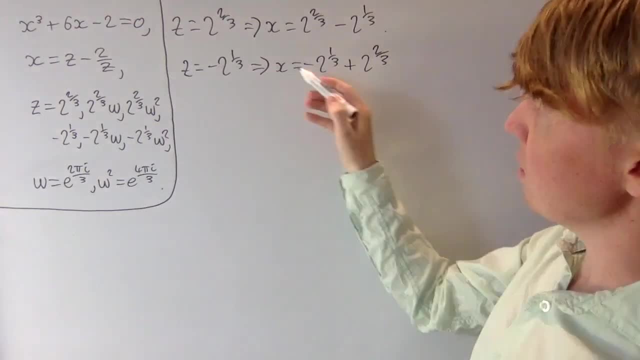 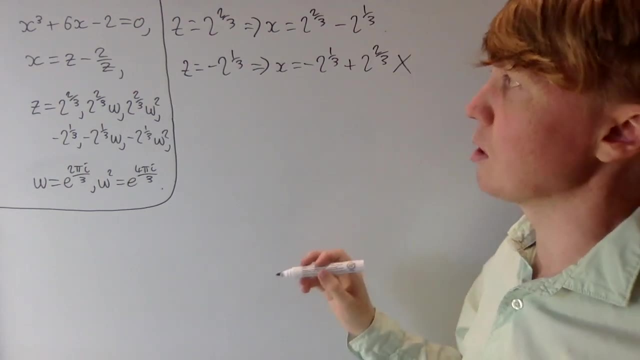 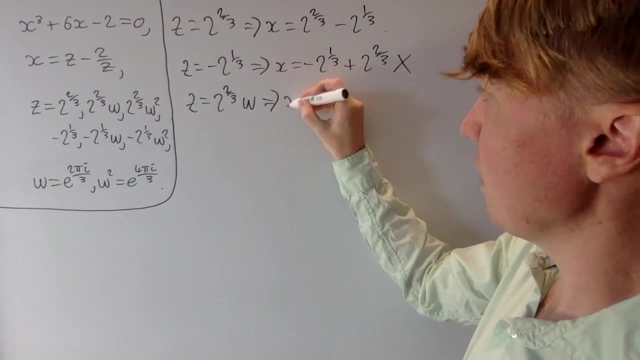 to the two thirds, and this is really interesting. you see, this is actually the same solution as we had earlier. so, even though we've got six potential solutions for z, we seem to be getting some repeats here, which is nice, so we'll move on now to. z is two to the two thirds times w. this tells us, then, that x is going to be two to the two thirds. 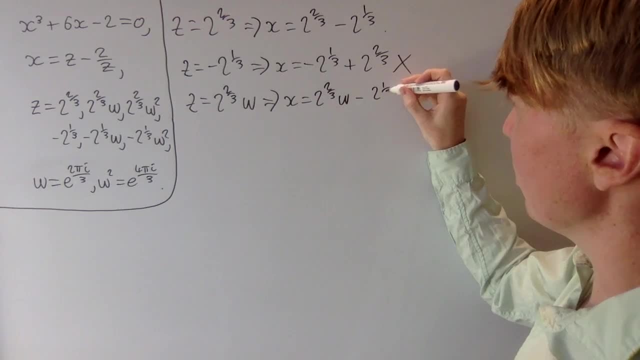 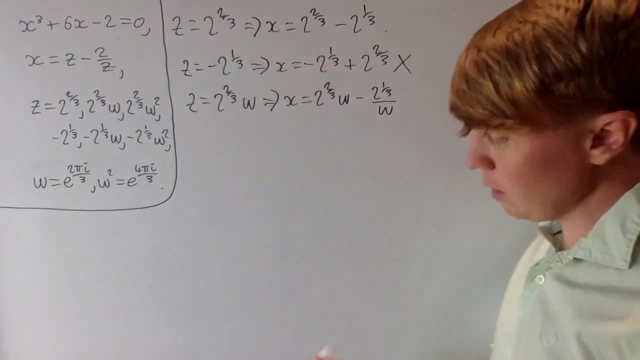 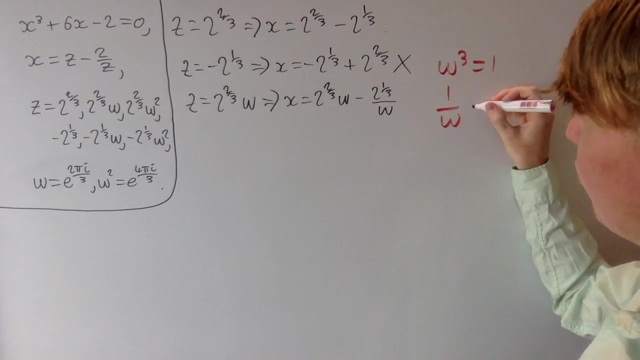 w. then we end up with minus two to the third over w when we do two over two to the two thirds w, and there's something really nice we can do here, because remember that w is a cube root of unity, so cubed is equal to 1 and a consequence of this is that 1 over w you can actually 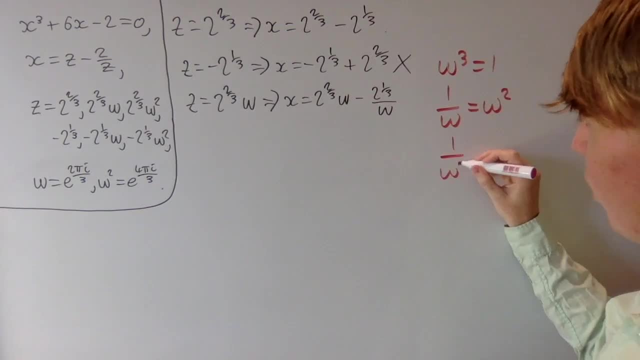 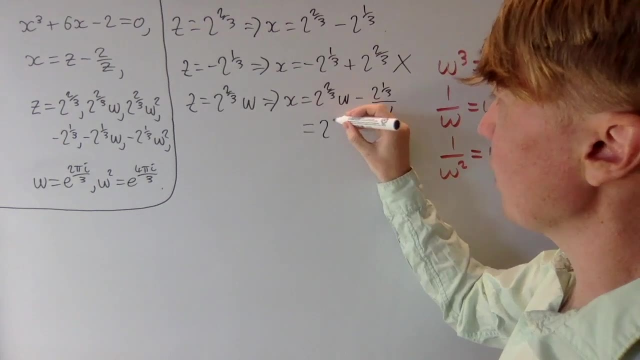 write as w squared, and similarly we can show that 1 over w squared is just equal to w. so this gives us a nice way of expressing our final solutions for x. here you get 2 to the 2 thirds w, minus 2 to the 1 third times w squared. so this: 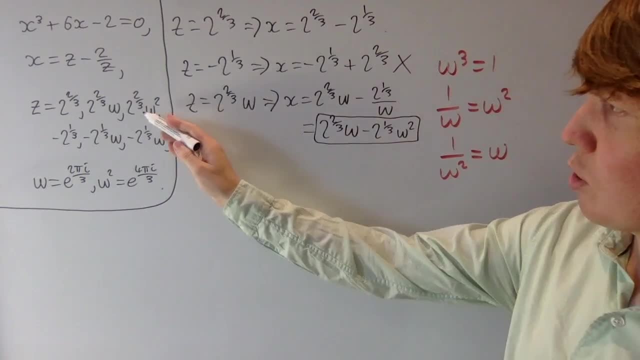 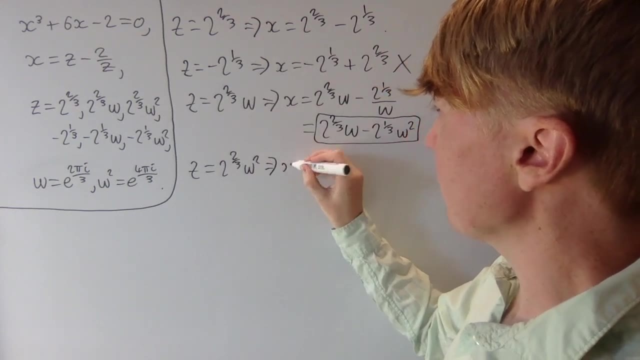 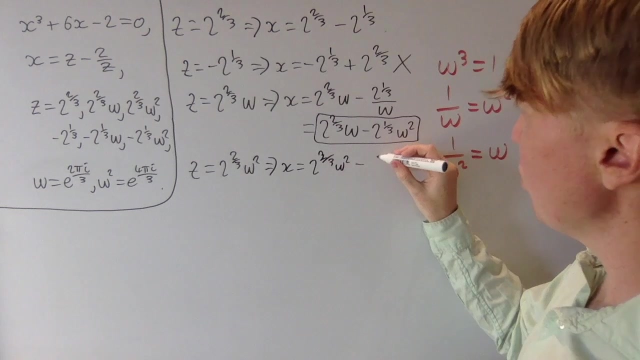 is our next solution. for x, we'll move on to 2 to the 2 thirds times w squared. so when z is 2 to the 2 thirds w squared, we see that x is going to be 2 to the 2 thirds w squared. then we end up with minus 2 to the 3rd over w squared. so 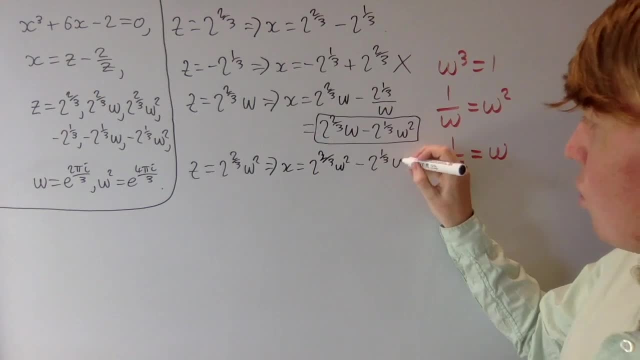 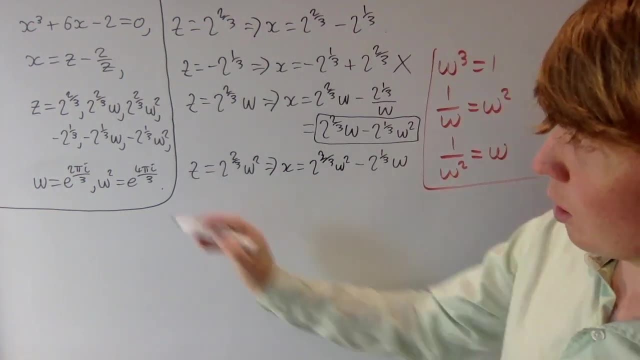 minus 2 to the 3rd, but 1 over w squared is just equal to w, so we can just write this with minus 2 to the 3rd times w moving on to our remaining ones here we could actually stop at this point, because we found this is a cubic. 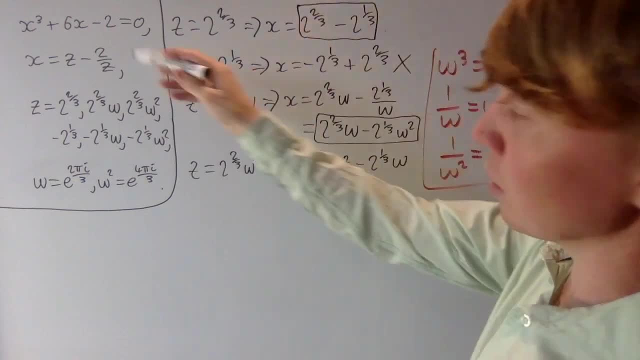 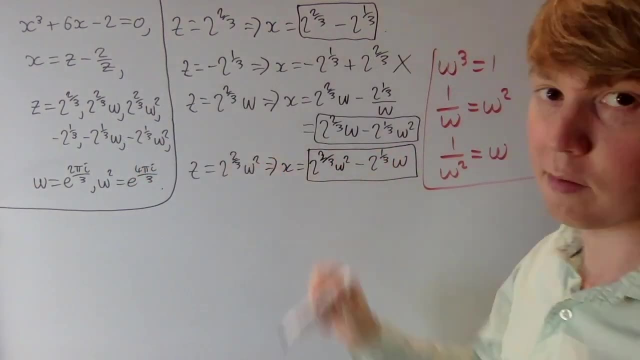 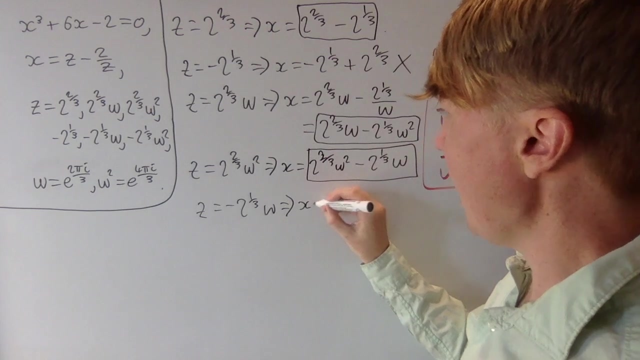 equation and we found 3 distinct solutions. we know that a cubic can have at most 3 solutions, but just for interest we'll have a look at what the remaining solutions are when we plug in these values of z. so z is minus 2 to the 3rd w this would give us. x is equal. 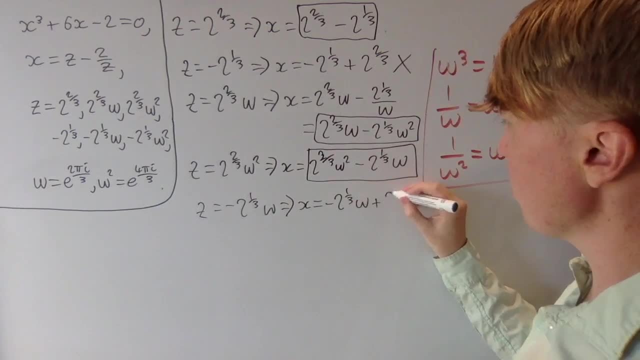 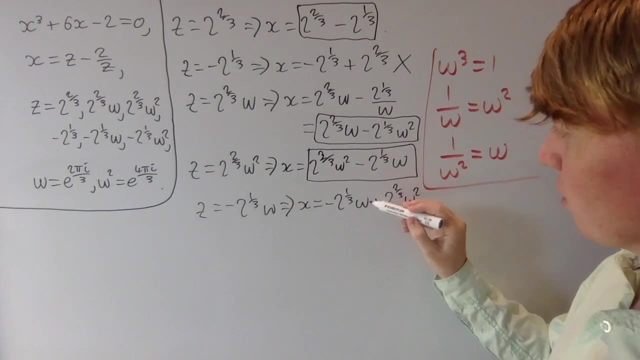 to minus 2 to the 3rd w and plus 2 to the 2 thirds times 1 over w, so this turns into a w squared. you see here this is actually just a repeat of the previous root that we've had there, so we don't need that one. and similarly, when we do z. 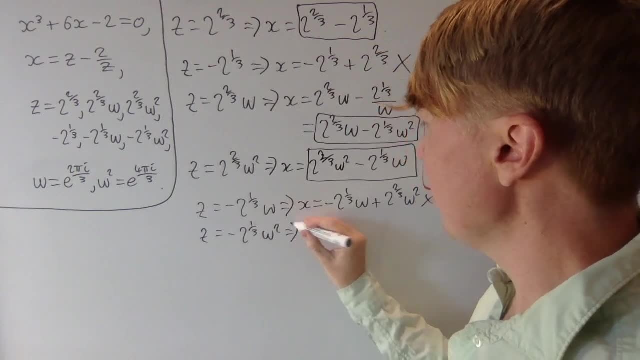 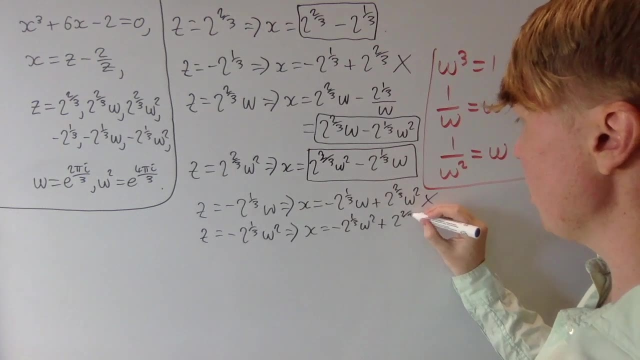 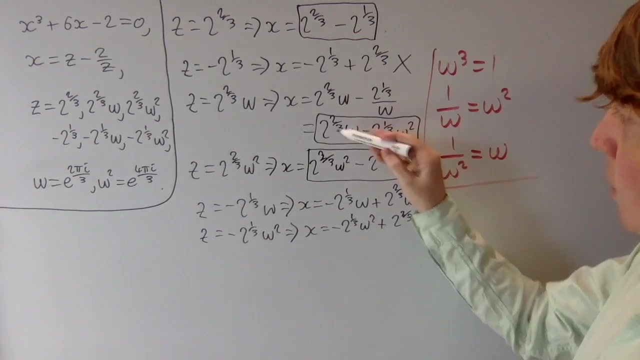 is minus 2 to the 3rd times w squared we get. x is equal to minus 2 to the 3rd w squared, plus we get 2 to the 2 thirds and the 1 over w squared just turns into a w. so we just have 2 to the 2 thirds times w. we see this is a repeat of our. 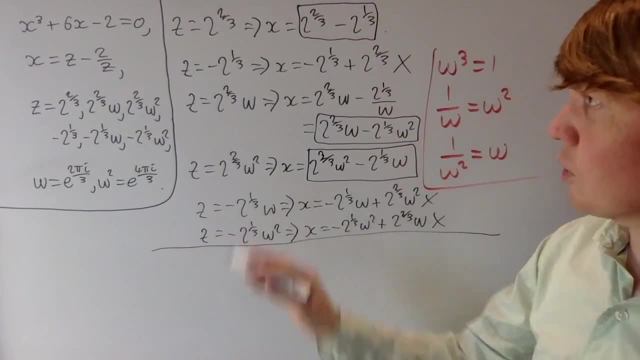 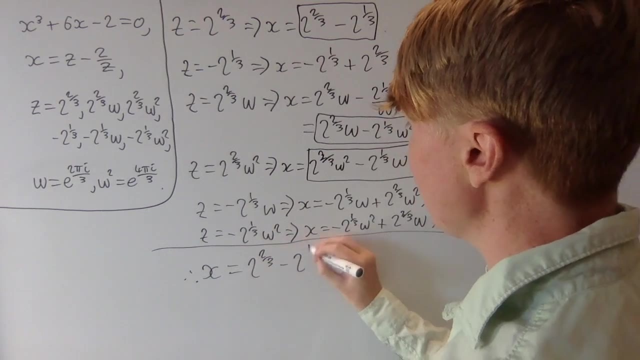 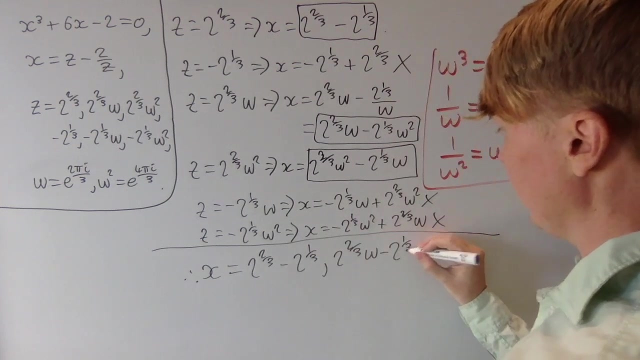 second root that we found there, so we don't need that either. so we've solved problem. now we can show that x is equal to 2 to the two-thirds minus 2 to the one-third. then it's also equal to 2 to the two-thirds w minus 2 to the third w squared. and your third. 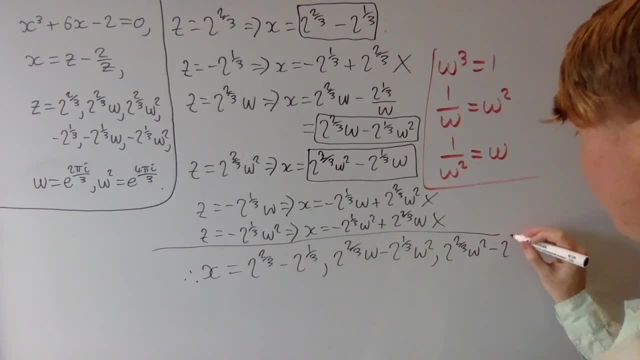 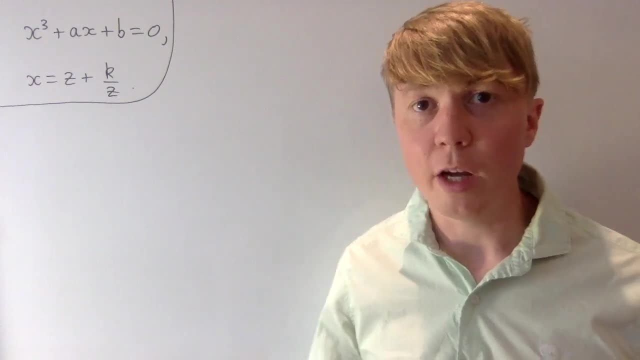 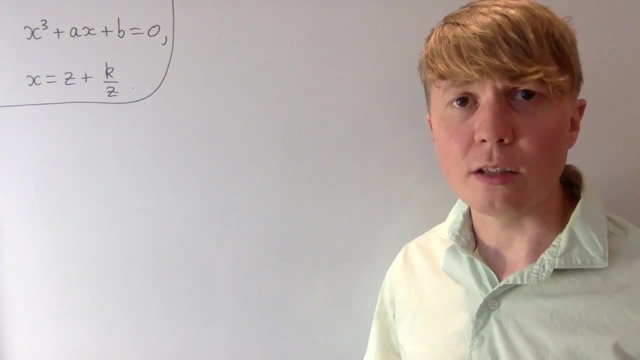 solution is 2 to the two-thirds w squared, minus 2 to the third times w. So how did we know that this substitution, this change of variables from x to z, was going to be helpful? And, more importantly, can we apply this method more generally? Well, this method is called Vieta's. 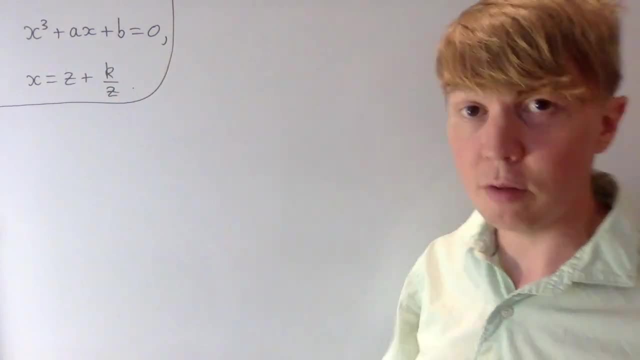 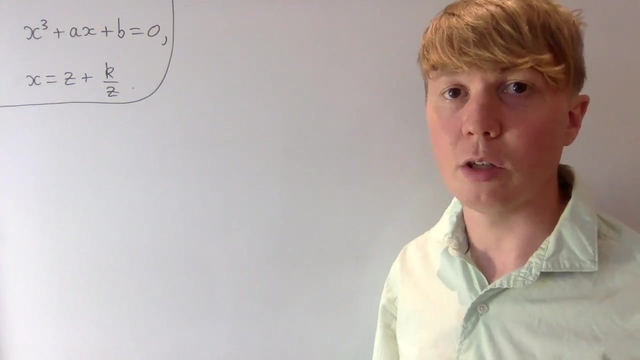 substitution, and this relies on having our cubic in this form, where your coefficient of x cubed is 1 and your coefficient of x squared is 0.. Unfortunately, there is a way to take any cubic equation and transform it by changing variables, so similar to how we replaced our x with z's. 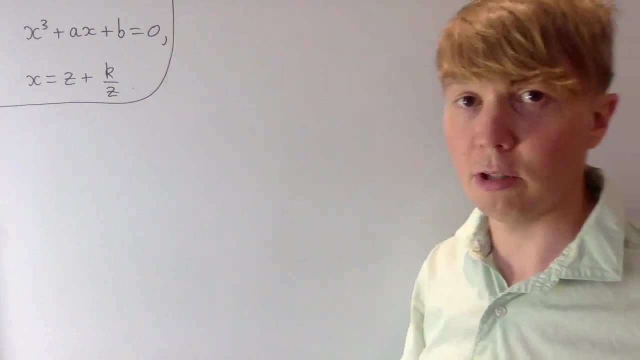 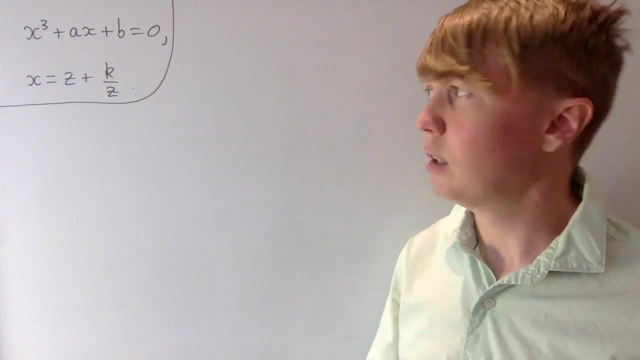 There's a way of taking any cubic equation and getting it into this form, so I'll include a link on that. So this tells us, then, that this method can actually be applied to any cubic, perhaps with a little bit of extra work. So then, the key idea here is we replace x by z plus k over z, and then this turns things into: 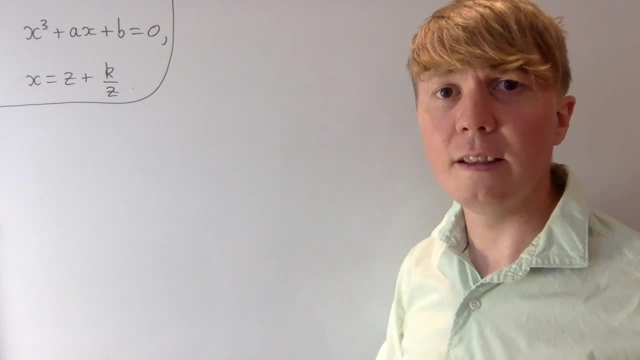 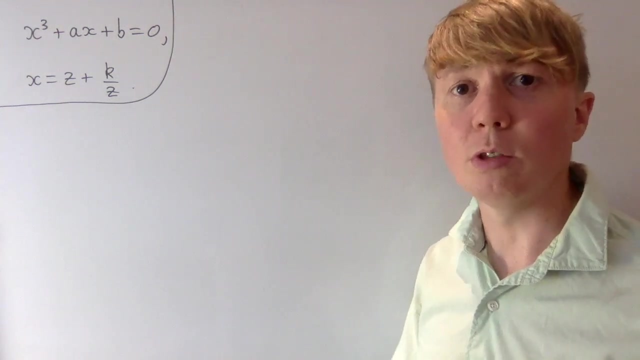 a degree six equation in z, And the idea is to use a clever choice of k which will turn this into something that's actually a quadratic in z cubed, which we can then solve to find z cubed. then we can find z, then we can find x. So let me explain what we mean here. We'll start off just by: 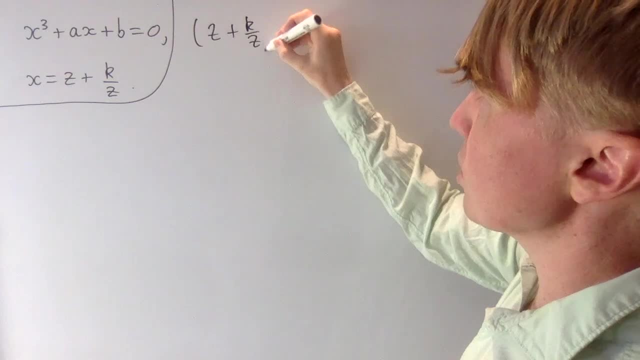 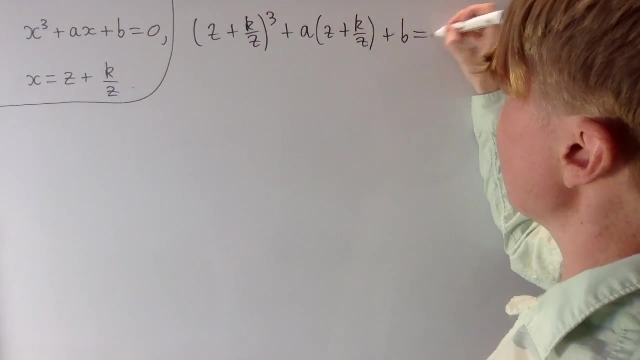 replacing our x's by z plus k over z, then we'll see what choice of k we need to make. So, plus a, z plus k over z plus b, all of this is equal to zero. So then, when we expand brackets, z cubed plus. 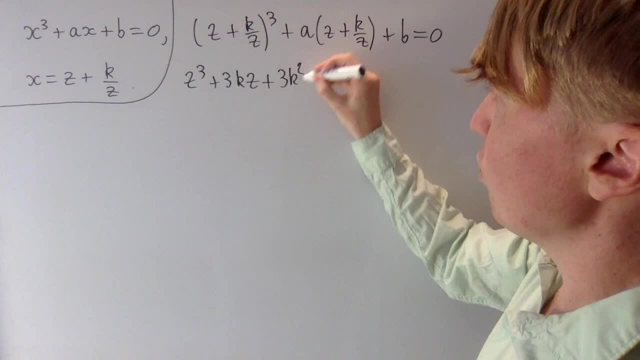 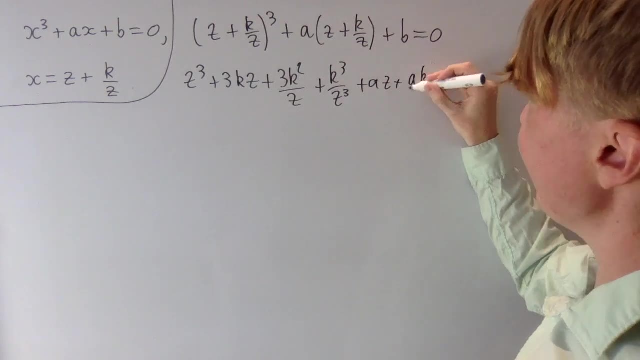 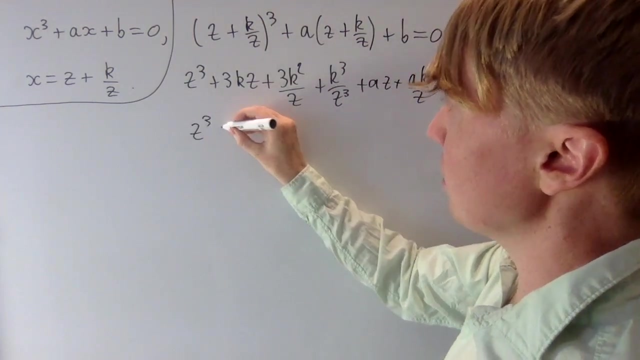 3k, z plus 3k, squared over z plus k, cubed over z cubed plus a, z plus a k over z plus b, this is equal to zero. So we'll collect our like terms, our different powers of z, so you get z cubed plus. 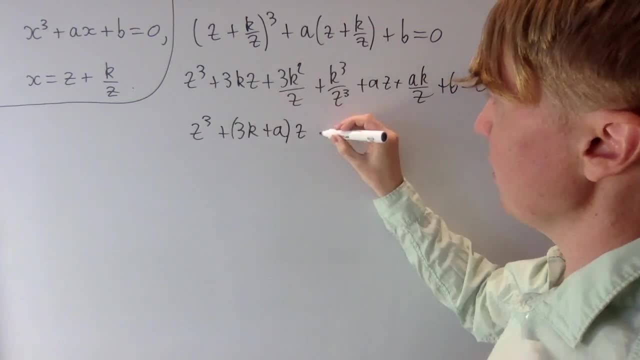 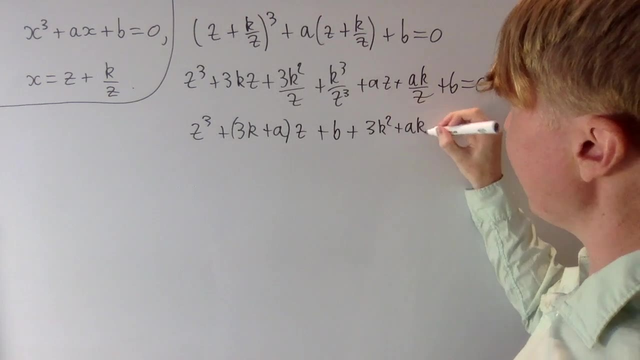 3k plus a times z, then we'll put the b term here in the middle. Then for our one over z's we get 3k squared plus a k all over z and then finally plus our k cubed over z, cubed term. so this is equal. 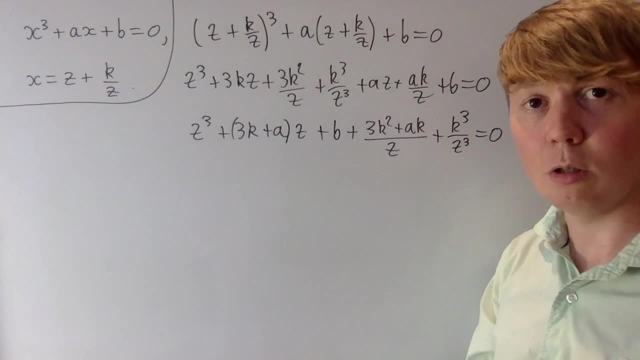 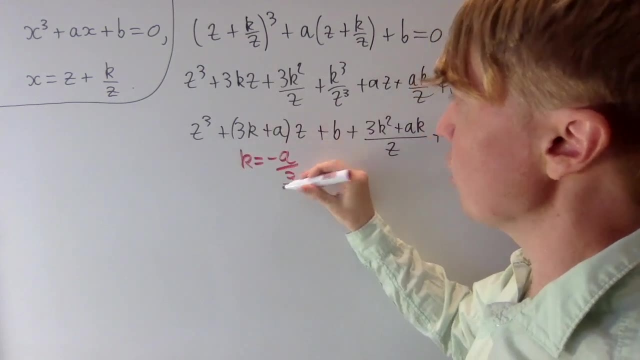 to zero, And what we'll do at this point so that we can turn this into a quadratic that we can solve. we want to get rid of this term here, so we're going to choose k equal to minus a over three, so that this vanishes. And, crucially, this is telling us then that our substitution is x. 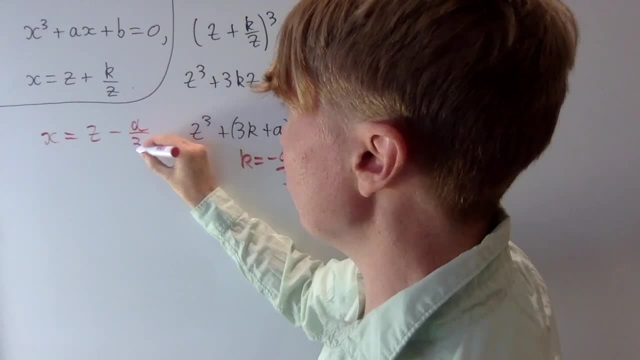 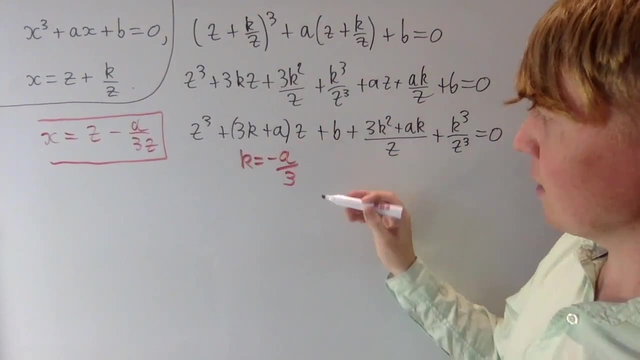 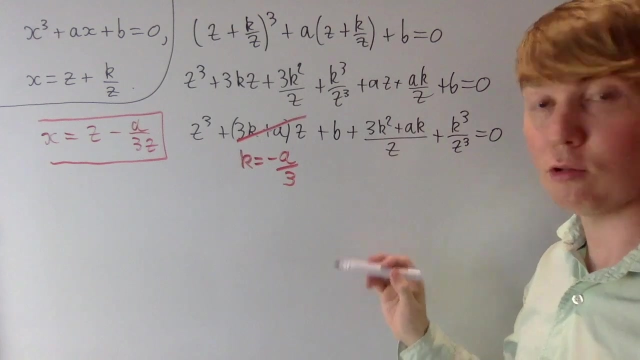 is equal to z minus a over 3z. So this is the actual substitution that we need to make here for this cubic equation. So this is really nice: When k is minus a over 3, this term disappears. What's really important as well is that actually, if you substitute in k is minus a over 3 into 3k. 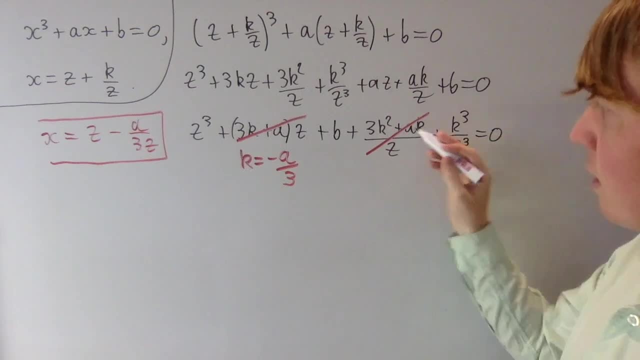 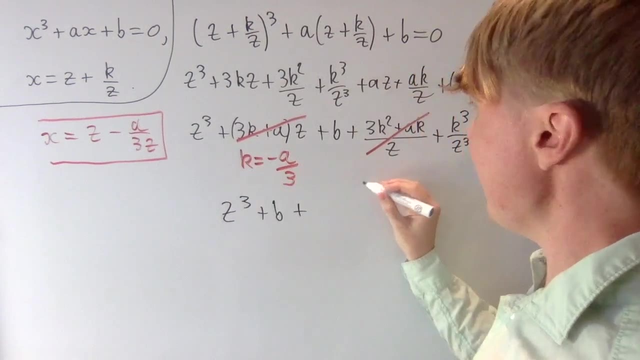 squared plus ak, this term actually disappears as well, and this is equal to 0, which is really nice, because now we just get z cubed plus b plus k cubed over z cubed. This is equal to 0.. So now, 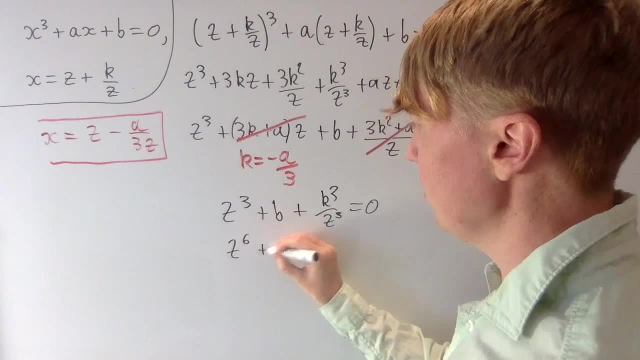 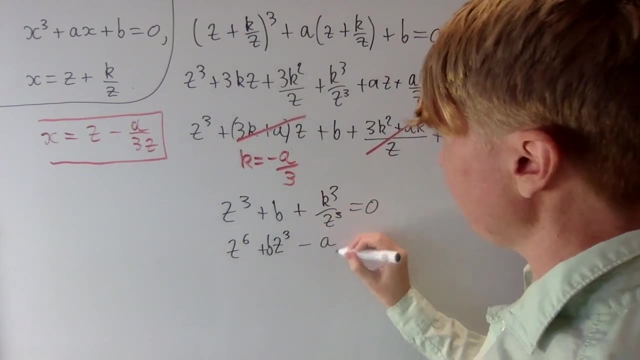 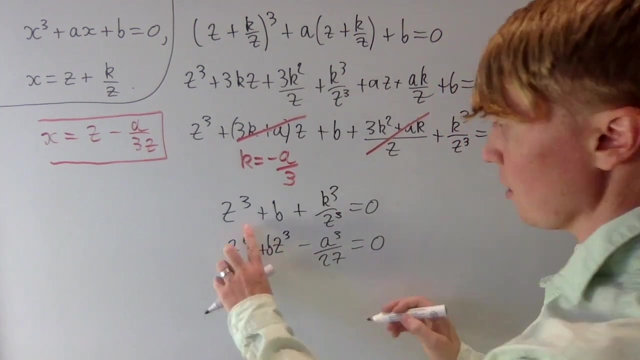 if we multiply by z cubed, we get z to the 6, plus z cubed times b, and we'll replace the k cubed by now, minus a cubed over 3 cubed, so 27.. All of this is equal to 0, and you can see here that z to the 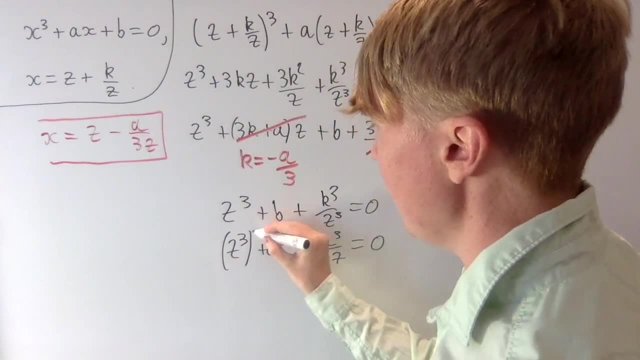 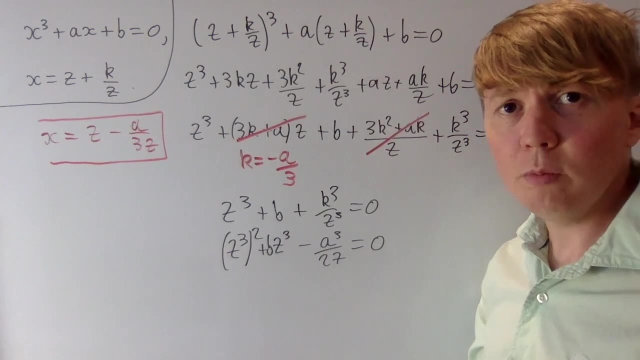 6, we write this once again as z cubed Squared. we've got a quadratic which we can solve to find z cubed, then we can find z, then we can find x. So the only problem at this point is we're going to get six possible solutions for z and we 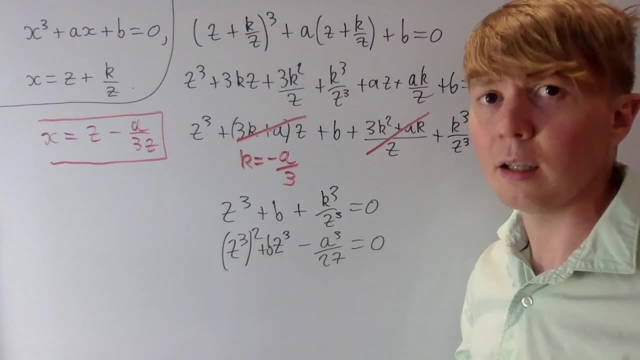 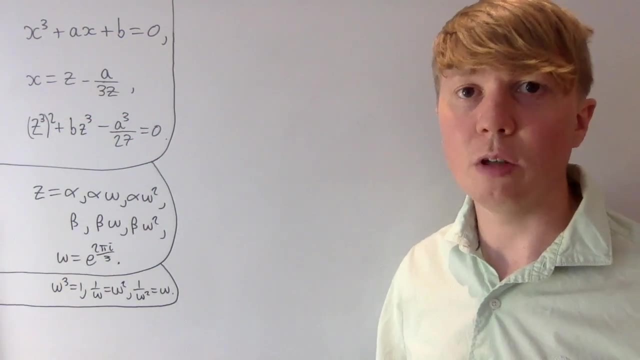 can only actually have three possible solutions for x when it's a cubic, so we'll explore this in a bit more detail now. So when we solve to find the values of z cubed, we can get up to two potentially complex solutions for z cubed. Then, working like before, we can take cube roots and we'll get a solution. z is alpha, but then if we solve to find the values of z cubed, we can get a solution. z is alpha, but then if we solve to find the values of z cubed, we can get up to two. 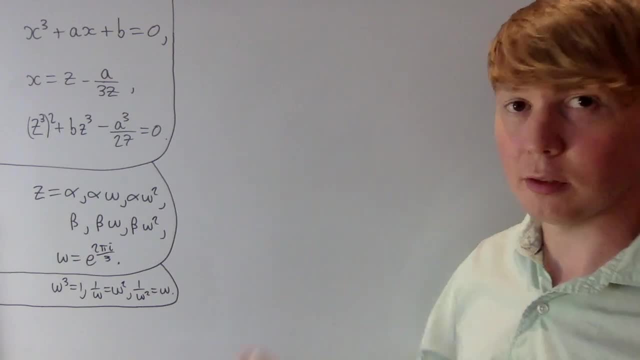 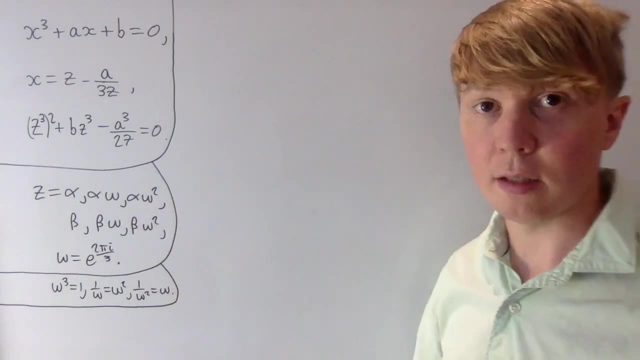 And if this is a valid solution, so will be alpha times w and alpha times w squared as well. If we've got another solution- beta when we take cube roots- we'll have beta times w and beta times w squared will also be solutions, And it's really worth emphasizing at this point that we're 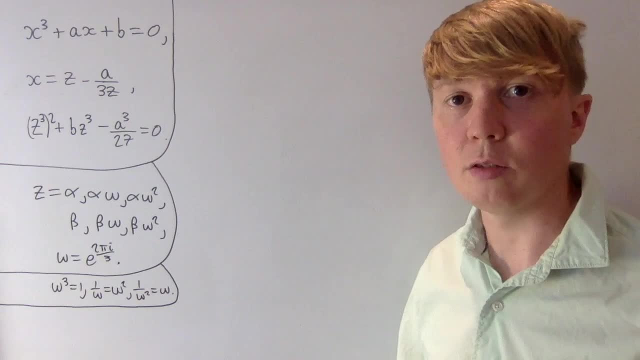 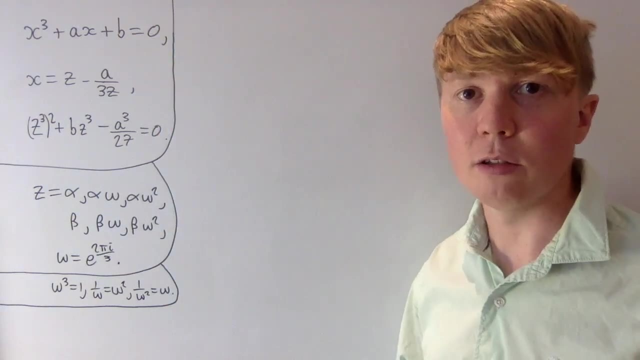 not actually going to get six distinct solutions here. there's going to be some repetition, which is really important because otherwise the method doesn't quite seem to work, where you need to get at most three solutions for x. So how can we see this? Well, we're going to use Vieta's. 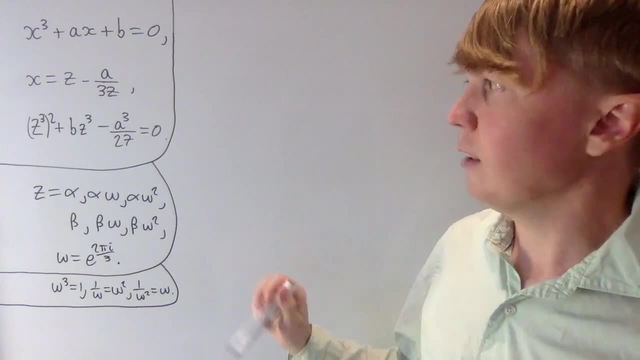 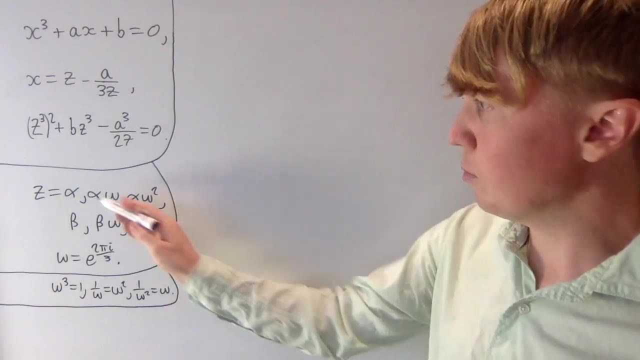 formula. We've got the six roots z here And basically we know that the product of the roots is going to be equal to minus a cubed over 27.. When we multiply together all of these roots, we'll actually just get alpha cubed times beta cubed. So don't forget that w cubed is equal to. 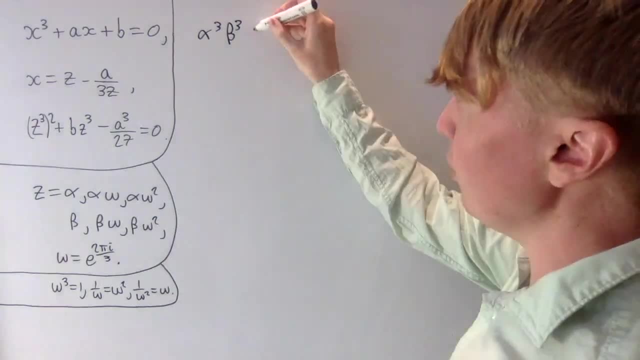 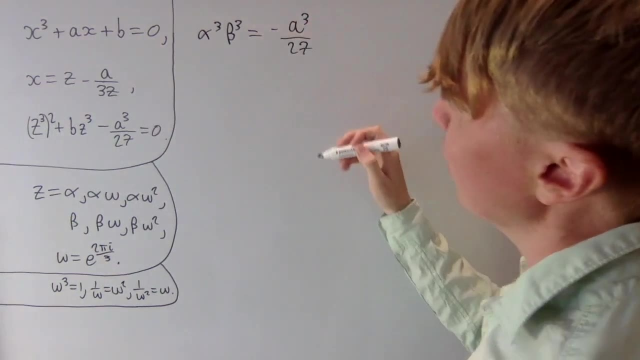 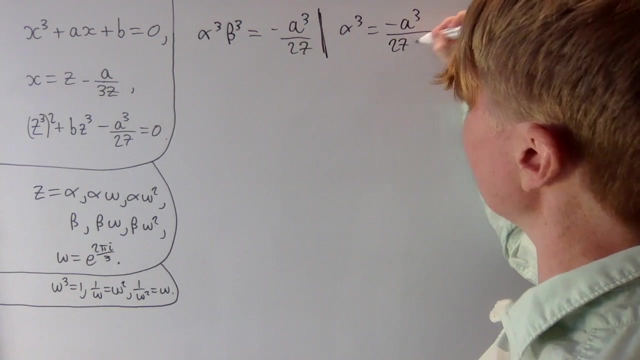 one. So these two lots of w cubed we get just disappear. So alpha cubed, beta cubed, using Vieta's formula, is equal to minus a cubed over 27.. And this is useful now, because let's just write this as alpha cubed is equal to minus a cubed over 27 beta cubed. Well, we don't know exactly what's going. 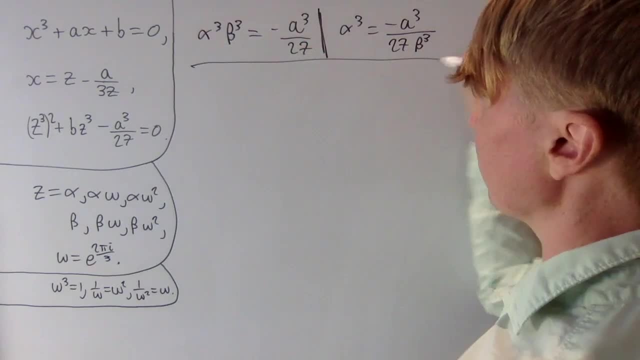 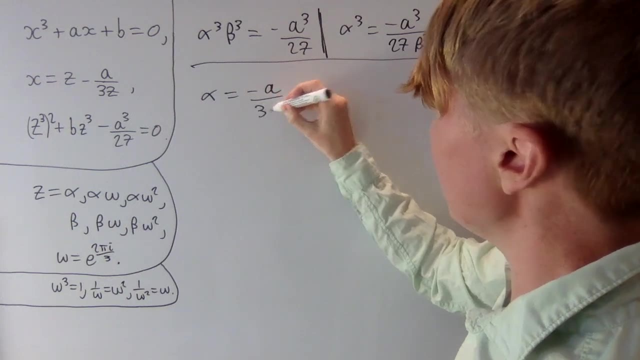 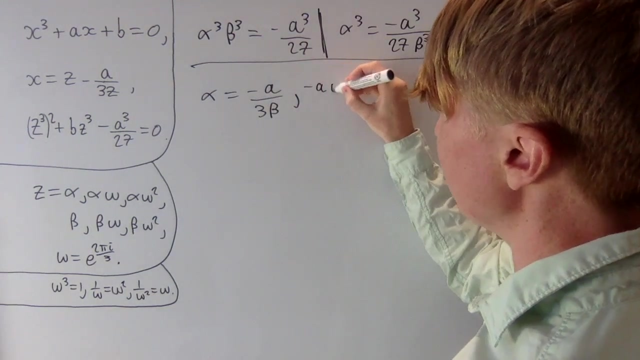 to happen when we take cube roots. but we can say one thing, which is that alpha is going to be one of three following options. So alpha is either going to be minus a over three times beta or, when we take the cube root of this, minus one. this is the problem really. you can have minus a w. 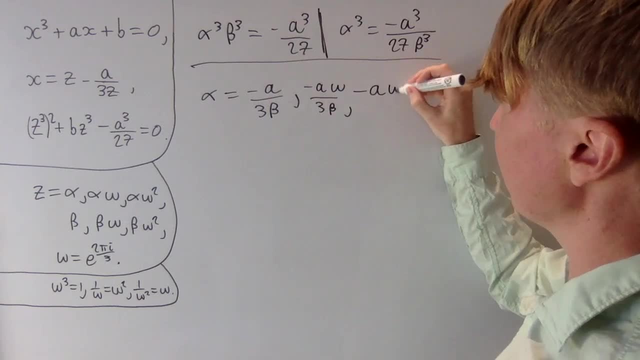 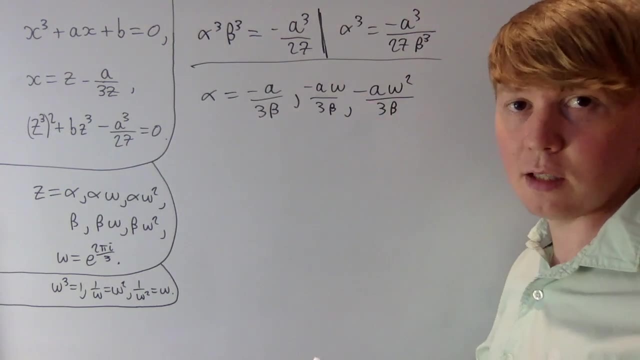 over three beta, or you could have minus a w squared over three beta. What we'll actually do as well here is we'll take these W's into the denominator. It makes sense in a moment why we're doing this, But don't forget w is equal to one. 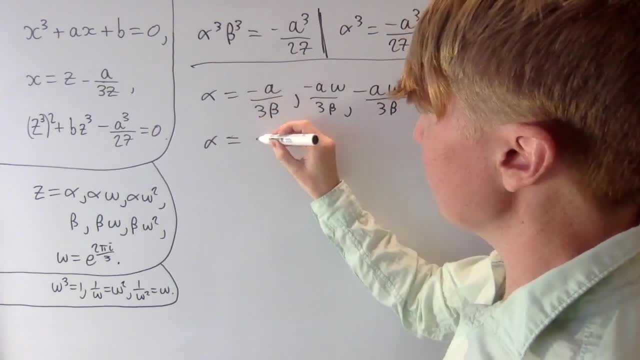 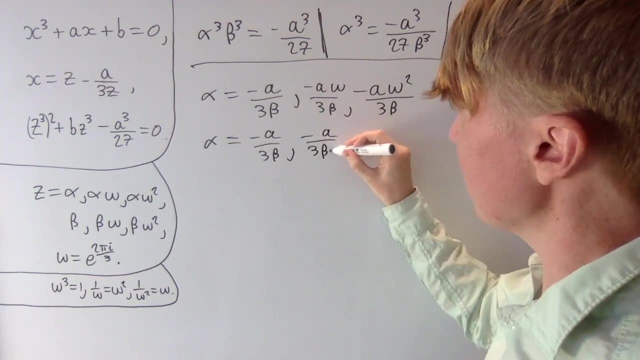 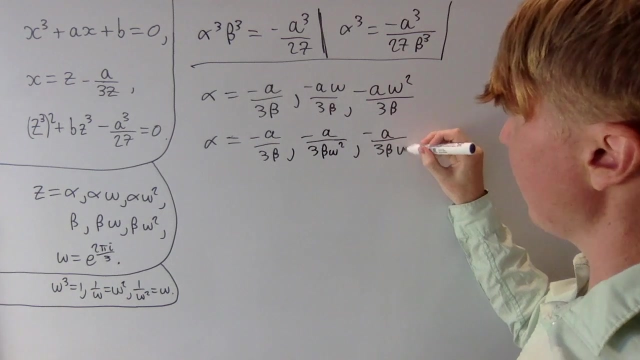 over w squared. So in each of these cases, alpha is equal to minus a over three b to begin with, or it's equal to minus a over three beta times w squared, or it's equal to minus a over three times beta times w, because w squared is equal to minus a over three times beta times w squared. 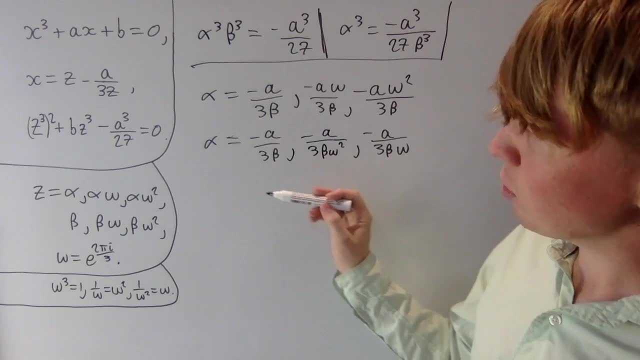 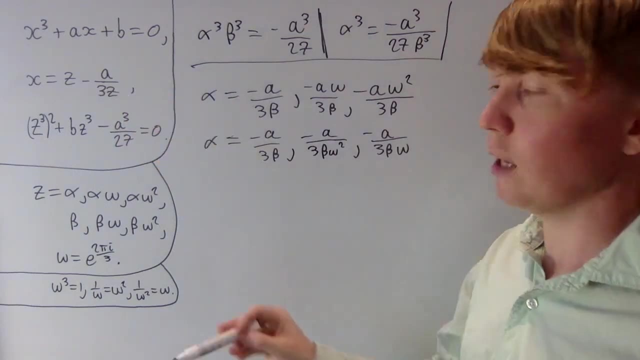 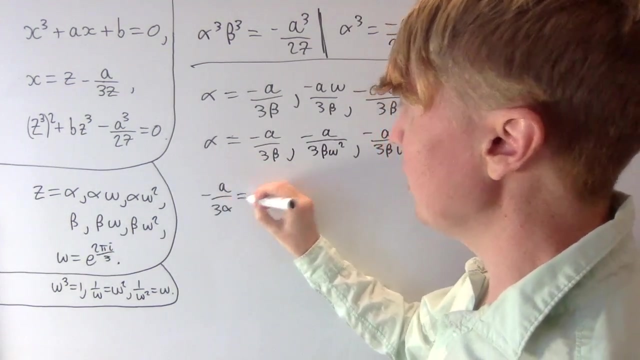 It's the same as one over w, So we're going to substitute these in. If you think z is equal to alpha, we'll substitute this in here: alpha minus a over three alpha to find our x solution. So we're actually interested in what is the value of minus a over three alpha in each of these cases. 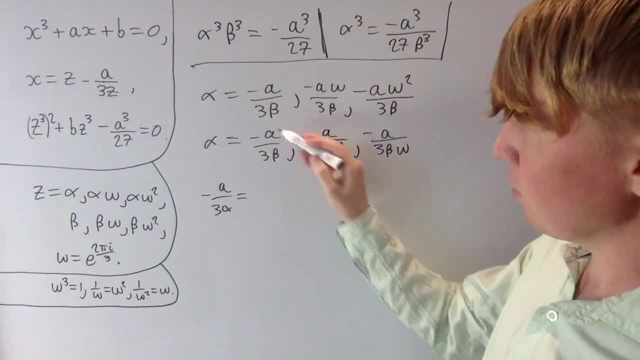 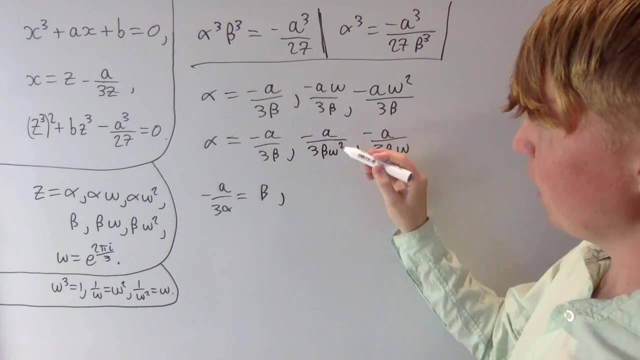 So when we take minus a over three alpha, when alpha is equal to minus a over three beta, we just get beta. And when we take minus a over three alpha, when alpha is equal to this, all we're going to get in the end is beta times w squared, and for this one, 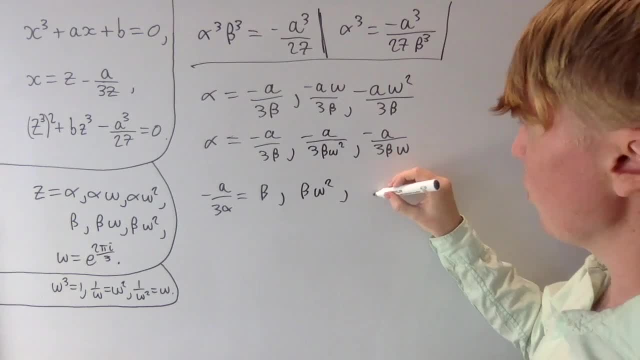 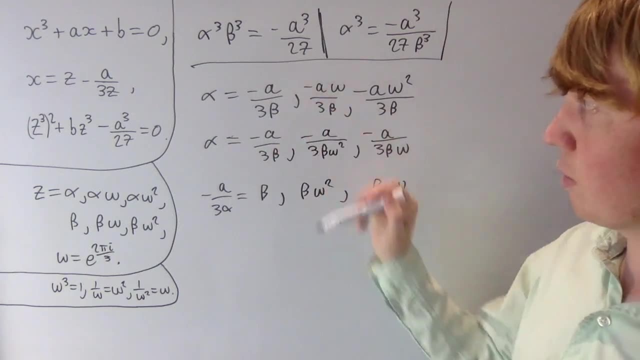 similar. minus a over 3 alpha is just equal to beta times w. so we don't necessarily know what alpha is equal to, but in each of these cases we know how to express alpha and a corresponding value for minus a over 3 alpha. so if we 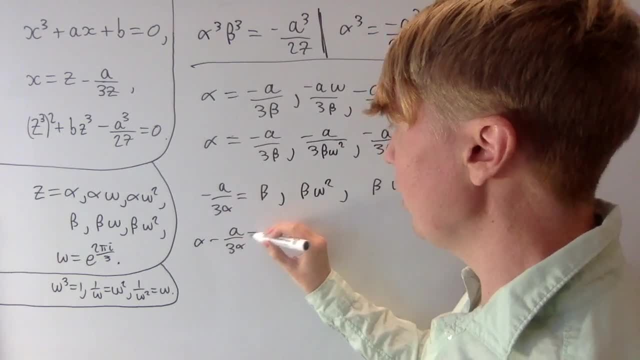 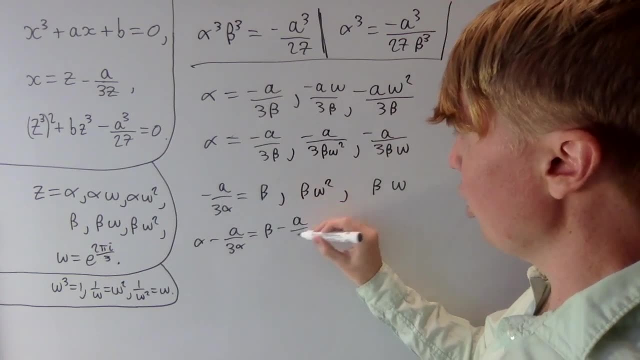 take alpha minus a over 3 alpha. what do we actually get? in each of these cases? you have minus a over 3 beta plus beta, so I'll write this as beta minus a over 3 beta in our first case, and then in the second case we'll have this term plus. 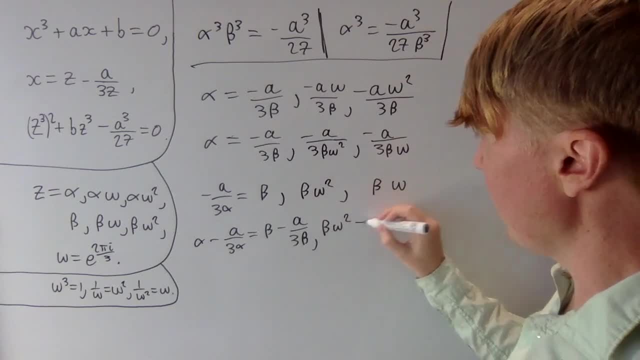 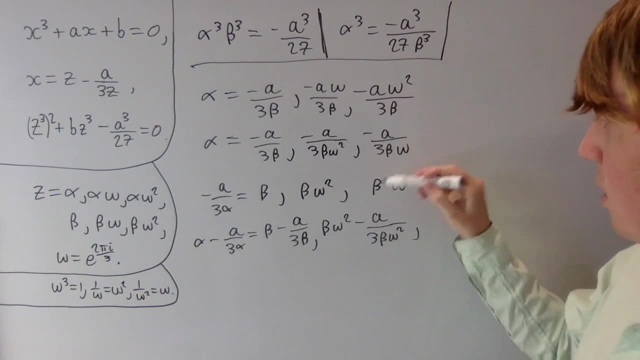 this term, so write this as beta w squared minus a over 3 beta times w squared. and finally, in our third case, we'll have this term plus this term, so write this as beta w minus a over 3 beta w. so this is really nicer, because you can actually see. we don't know which case we're in, but in each of these cases, 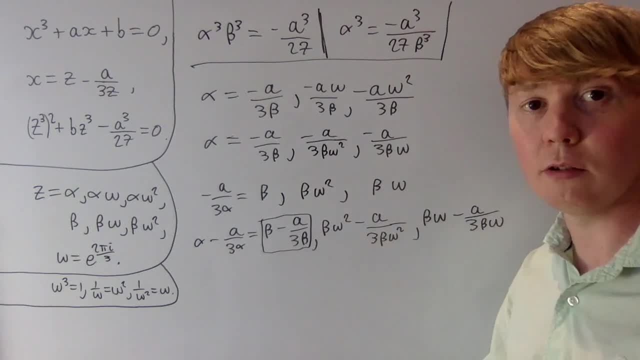 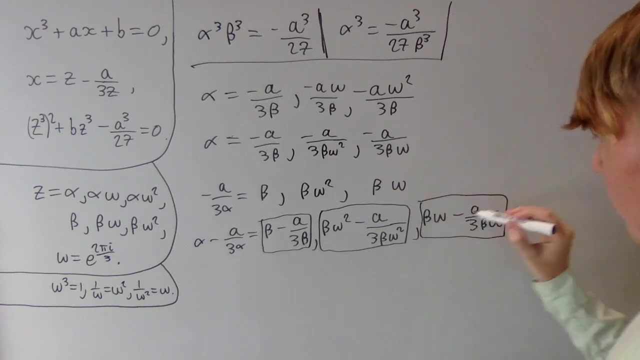 beta minus a over 3 beta. this is actually the x solution you would get if you took z equal to beta here, In this case, beta w squared minus a over 3 beta w squared. this is the x solution you would get if you took z equal to beta w squared. And finally, this one beta w minus a over 3 beta w. 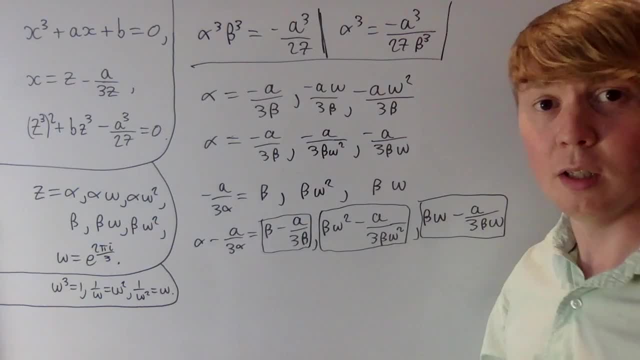 is the x solution you would get if you took z equal to beta w. So we're always going to get a duplication here. alpha minus 3 over alpha is actually the same as one of our beta solutions. So we can do something similar with alpha w and alpha w squared. 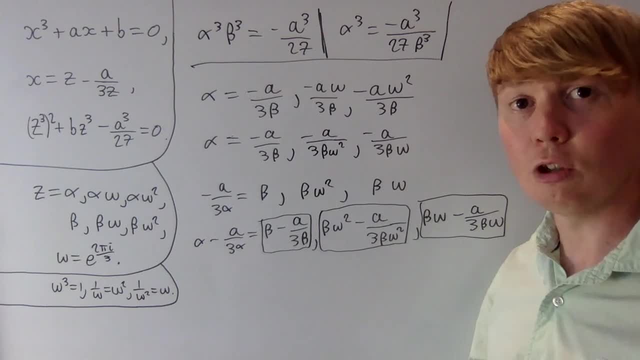 So this explains why we don't actually get six solutions. they're always going to come in pairs.